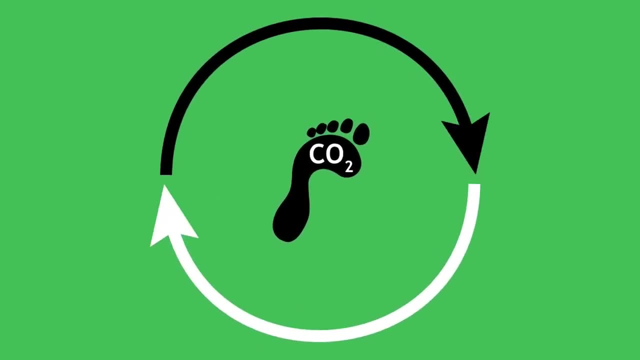 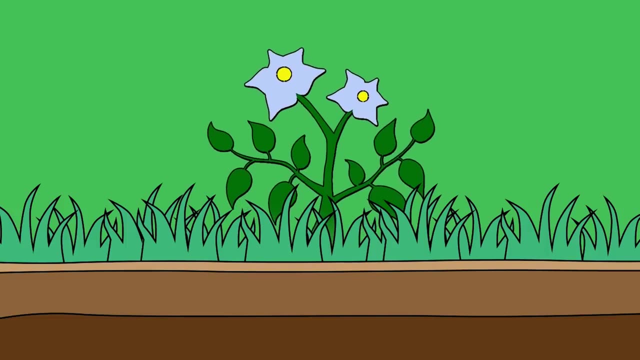 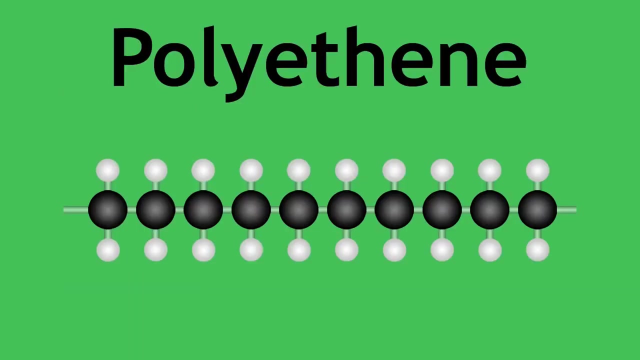 our environment, but a long term goal for many chemists is to develop more biodegradable plastics which would naturally break down in our environment. Here are some specific examples of polymers and their common uses: Polyethene, Used for carrier bags and sheet plastics. 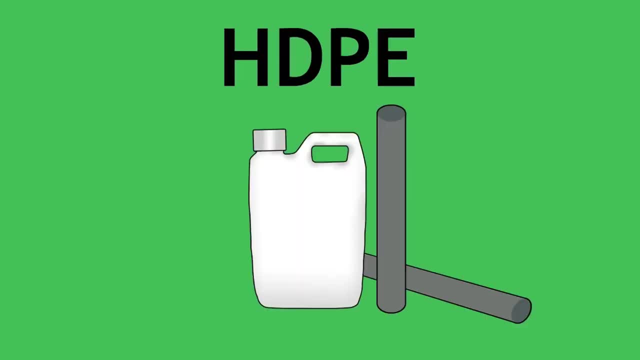 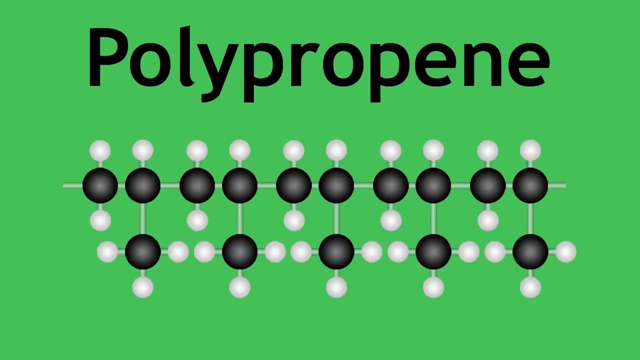 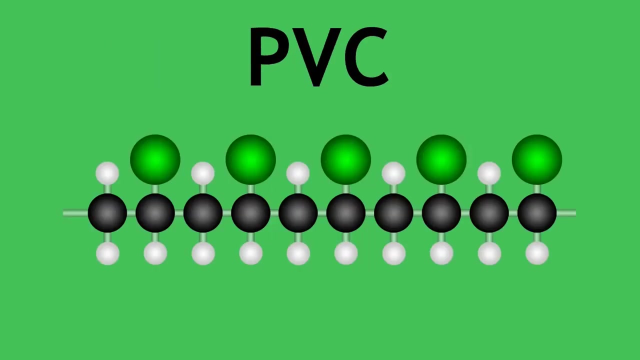 High density polyethene used for drain pipes, water bottles and containers. Polystyrene used in packaging. Polypropene used for bottle caps, plastic bottles and plastic pipes. Polychloroethene, often known as PVC, and is used for windows and doors. Polychloroethene is also used for windows. 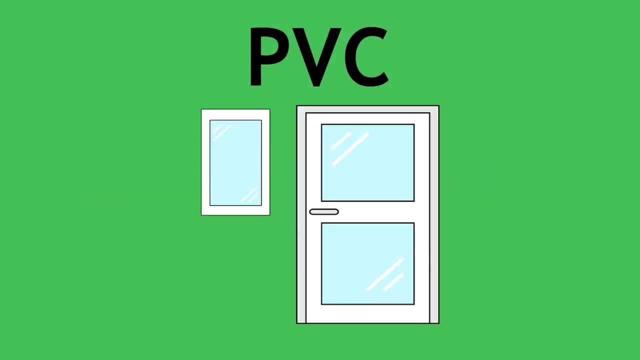 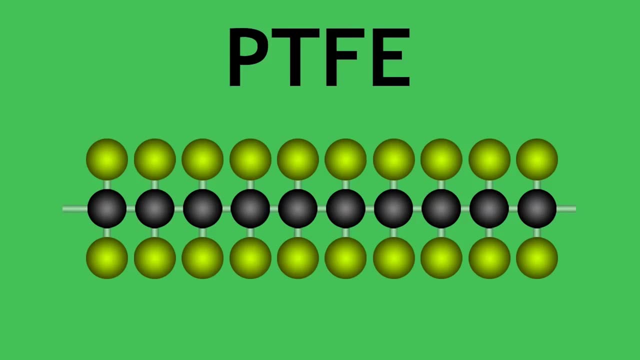 and doors. Polychloroethene is used for windows and doors. Polychloroethene is also used for frames, plastic hinges and bottles. Poly-1122 tetrafluoroethene, also known as PTFE, which. 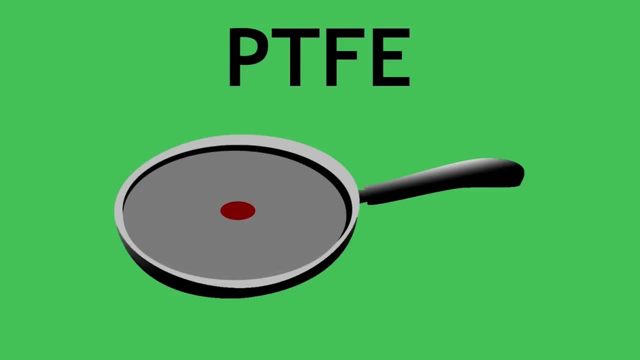 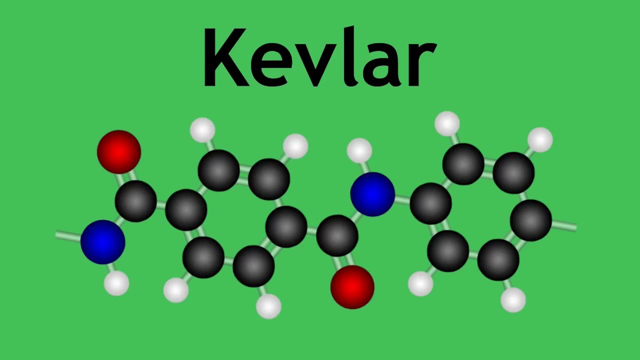 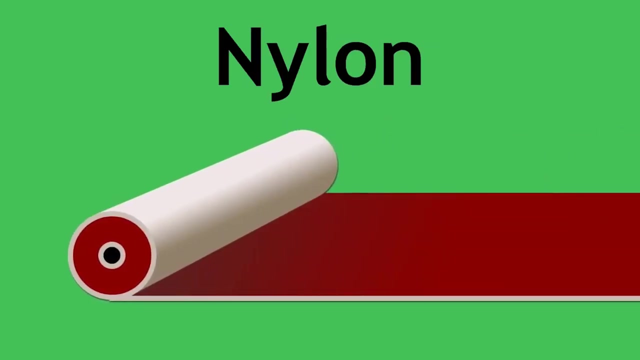 is a non-stick coating on frying pans, as well as being used in bearings and other low friction surfaces. Kevlar is a unique polymer in that it formed bulletproof vests and jackets. Nylon is used in textiles, clothing and carpets. As you can see, polymers play a huge role in our 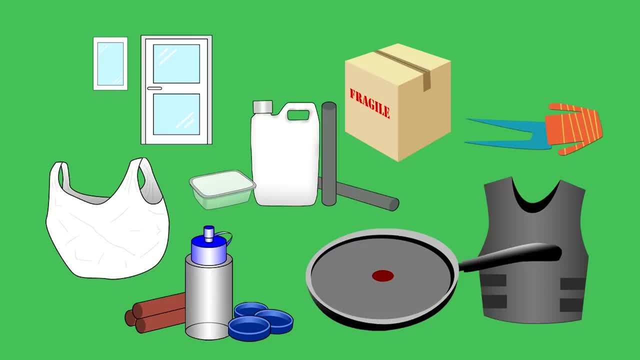 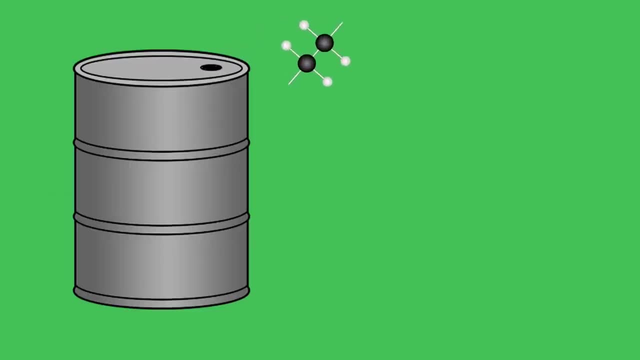 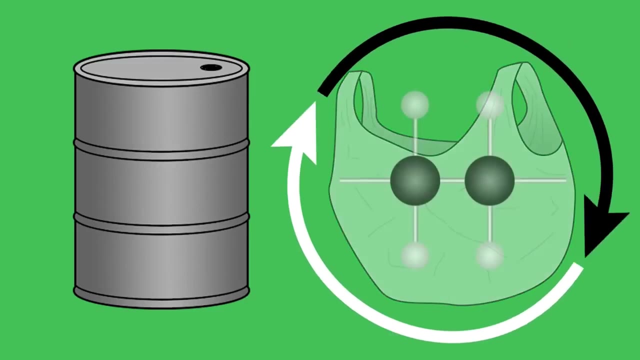 day-to-day lives, and their use is wide and varied owing to their unique individual properties. It is important to understand that most of the alkyl monomers used to make polymers are obtained in some part from crude oil, and therefore it is critical that we recycle plastics to 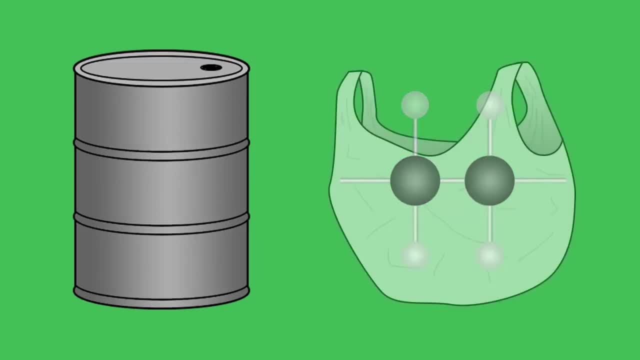 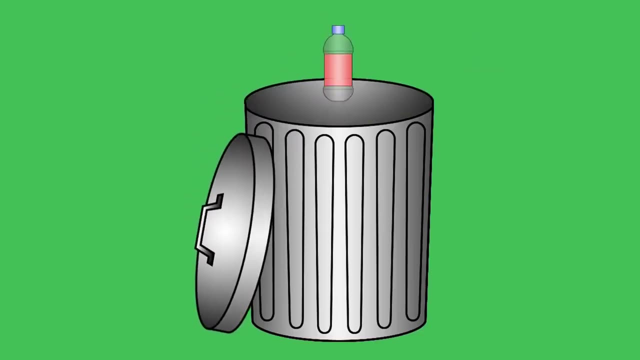 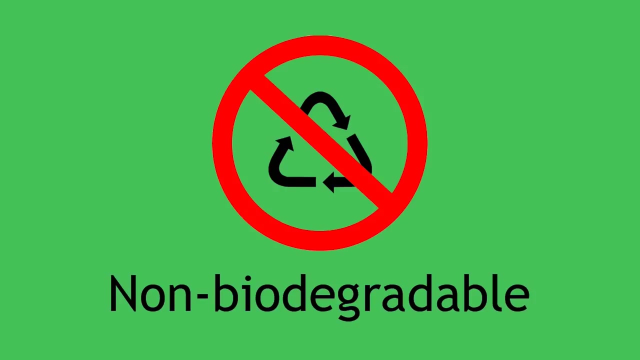 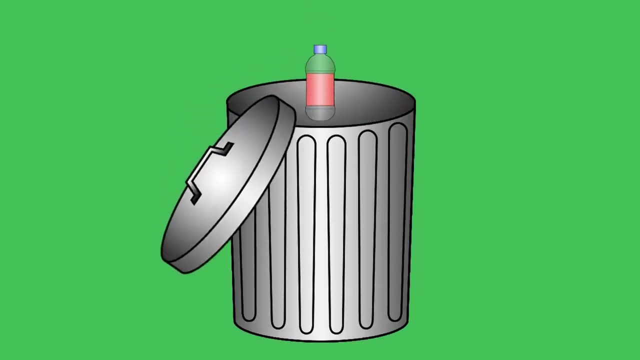 conserve our natural resources for the future manufacture of these polymers. There are also big problems associated with the disposal of polymers. The biggest problem, as mentioned above, is that polymers are non-biodegradable, which means that microorganisms cannot naturally break them down. Disposal of polymers by burning or incineration. 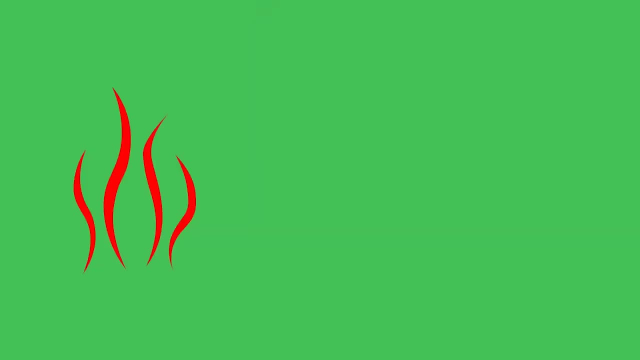 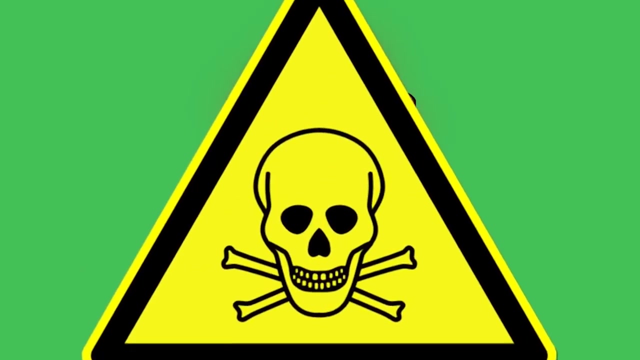 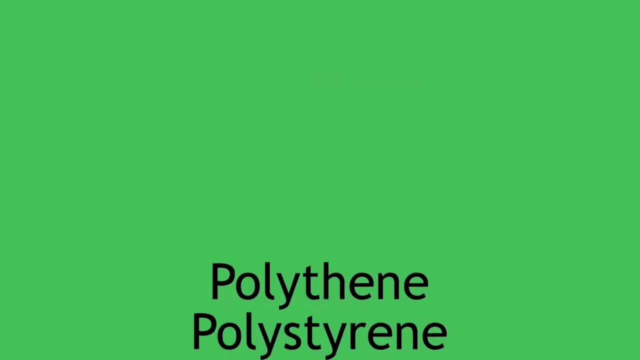 is a possibility, as this generates heat which can be used to generate electricity. However, the burning of polymers produces many toxic gases, which themselves can damage the environment and cause pollution. Now, at the end of this lesson, you should have an appreciation of